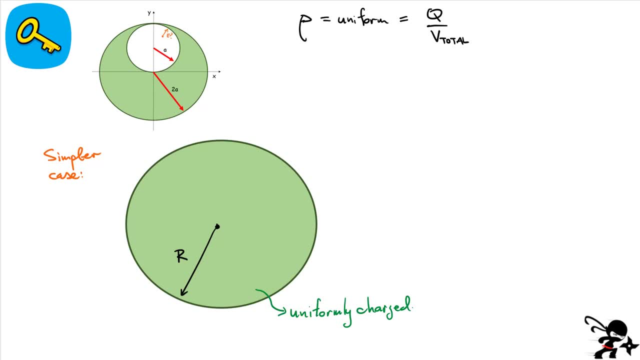 and the sphere has a radius big R and I want to apply Gauss's law to find the field inside that sphere. So Gauss's law says that the integral of E dot dA, that's over a closed surface, is equal to how much charge is inside my closed surface divided by epsilon zero. Now my goal is: 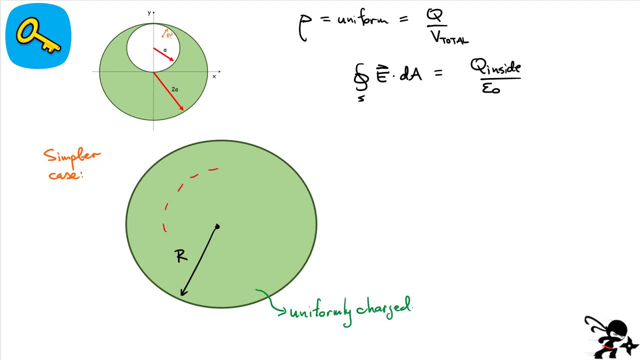 to find the field inside. So I would draw a Gaussian surface and I'll just show it here. Just sketch that quickly. This Gaussian surface has a radius little r, All right, so how do I apply this? Well, again, if you were going to draw 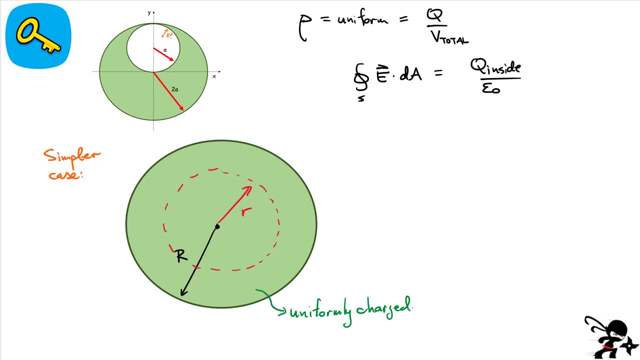 the electric field. at any point inside, on this Gaussian surface, the electric field would be pointing away if this object is positively charged. Now, because of this symmetry, what this does is it really simplifies the left-hand side here of Gauss's law, Because E is has a constant. 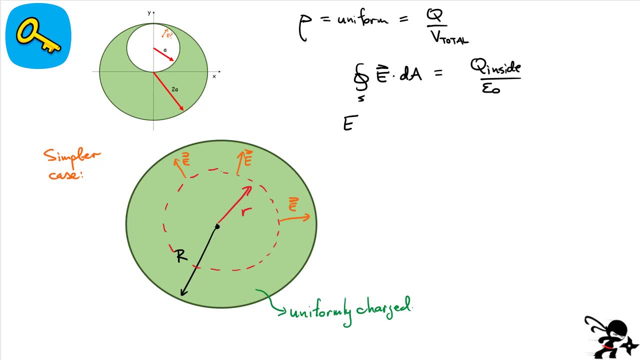 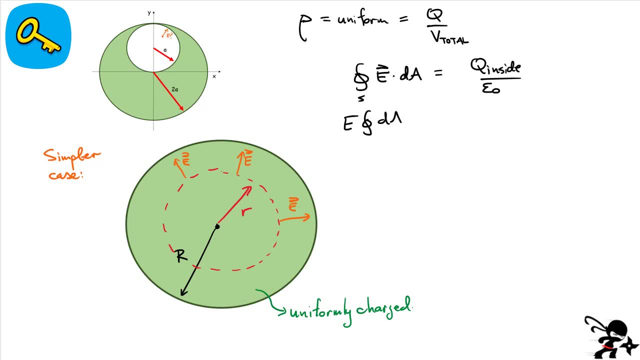 and you're left with the integral over a closed surface of dA, That is simply the total area of this sphere. All right, what about this left right-hand side of Gauss's law? It says Q inside. it's how much charge is inside this volume divided by a constant epsilon zero. So the charge inside. 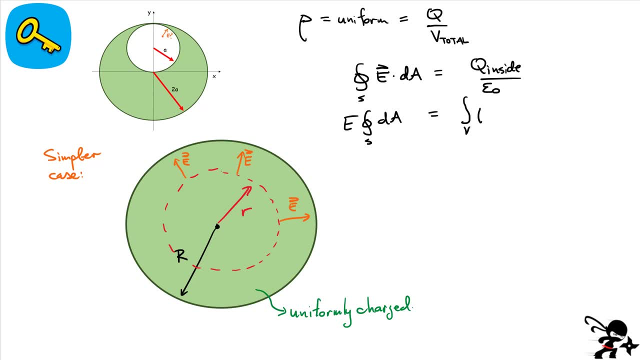 again, all you have to do now is integrate over the volume of the charge density over that volume. okay, divided by epsilon zero. So let's look at both sides again. So the left-hand side simplifies the integral of the area here, of this closed surface, gives me four pi little r. 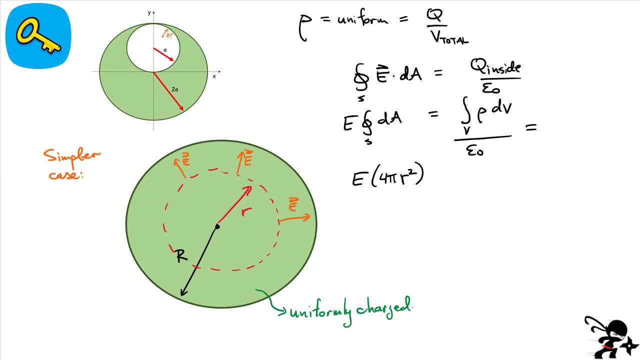 squared. That's the area of this surface of the sphere. All right, what about the right-hand side? Again, this numerator here simply boils down to again the density, and it's not just this part, but this whole area here. Now, this is going to be a little bit. 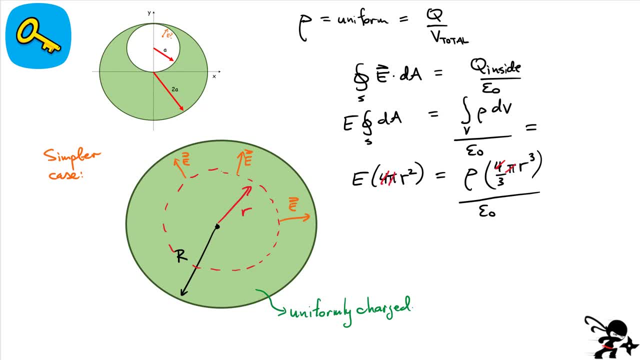 of a pain, the step-by-step way to do this. but you could simply take it out of the integral and you're left with the integral of the sphere. as for a little radius, and I could take it out of the integral And I'm left with integrating the total volume of this sphere, The total volume of 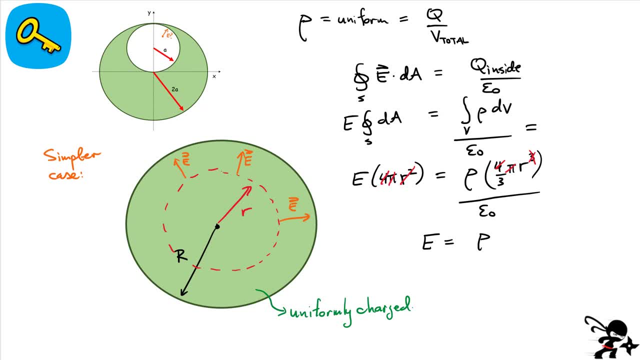 magnitude of that electric field is the density. I still have a 3 left over epsilon 0. I still have one value of r. That is the magnitude. If I wanted to write it as a vector, what you can do is just write e and then I can add a vector r, like this: Okay, so that tells me that the field 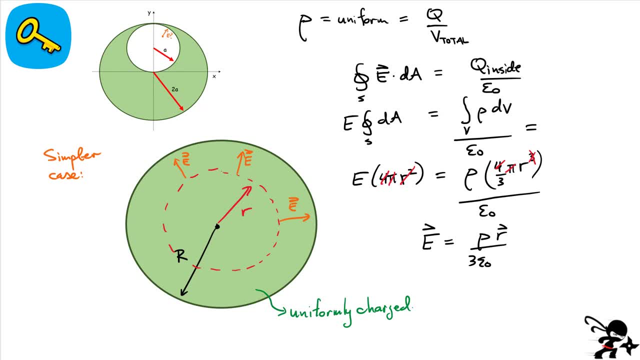 is radially pointing away from the center of the sphere. Okay, so we're going to use this result now in order to find the field of a much more complicated object- Okay, the object I have here above the object with a cavity inside. Let me show you the trick on how to do that. All right. 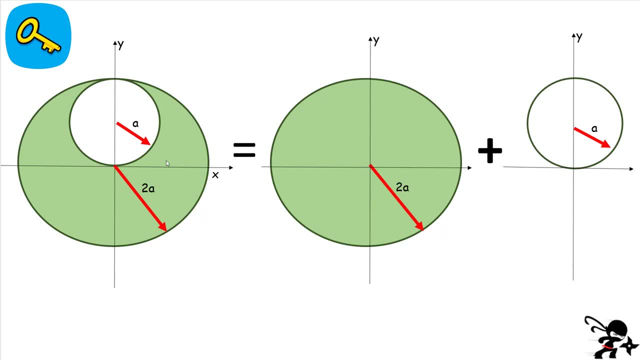 the second key to finding the field anywhere inside this cavity- all right, let's call that e inside or e total- is to use the principle of superposition. All right, let's think about from an electrical charge standpoint. how can we create an object like this? 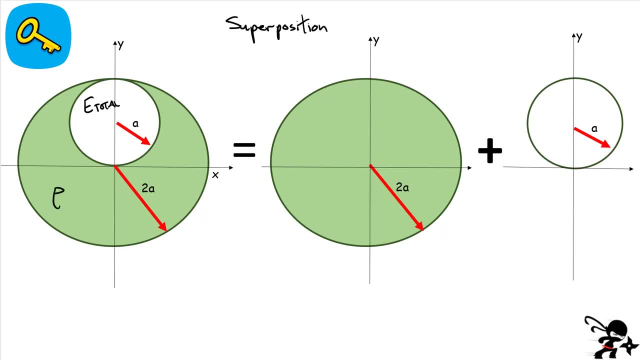 that has a charge density, rho, that is uniform everywhere in the green shaded area and is zero inside this white area. Well, this object can be made by considering a total sphere which has the same charge density as the first one and if I add to it something with an opposite charge density. 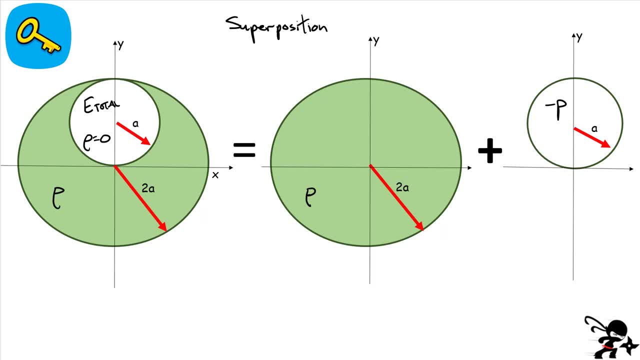 So at the end, if I put one object over the other, it is going to cancel the charge in such a way that there is no charge density. So if I put one object over the other, it is going to cancel the charge in such a way that there is no charge density. So at the end, if I put one object over the 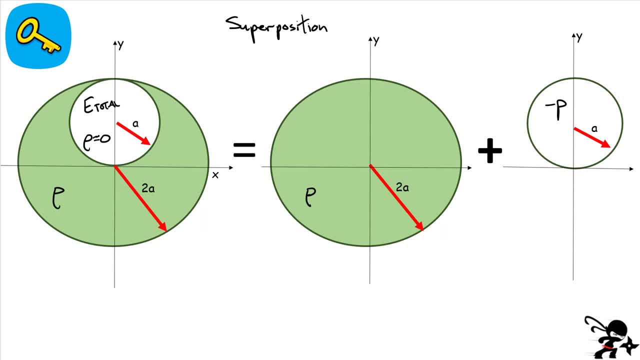 other, it is going to cancel the charge in such a way that there is no charge density. So at the end, if you consider it so, our total electric field, at any point, I would write it as a vector and I would write it as the field due to this positively charged object, right the full sphere, and to it. 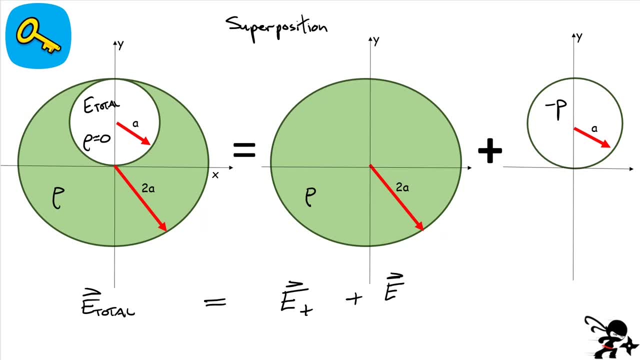 I would add the field produced by this negatively charged object. I'll call it e negative. This is the field, due to a small sphere, with a negative uniform charge density applied over its volume. Okay, so this is what we're going to do now and what we are going to end up. 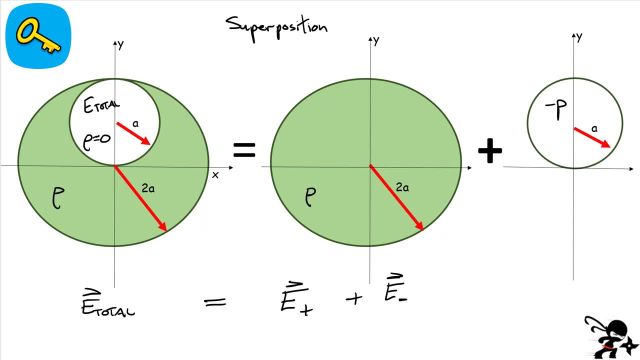 doing is: we're going to use the result from the previous case, we're going to use Gauss's law for this guy, and we're going to use Gauss's law for this guy in order to find the total electric field. So let's go on the next page and start putting things together. I'm considering an arbitrary. 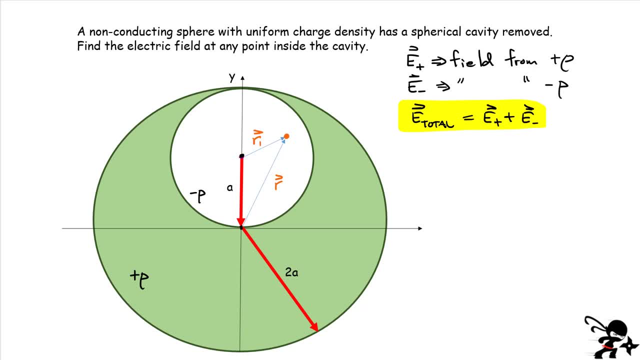 point anywhere inside this cavity. Okay now, this point I could define as a certain distance away from the big sphere or a certain distance away from the small sphere, and I'm going to use that for the different vectors that I'm considering. So, again, we have to use superposition to solve. 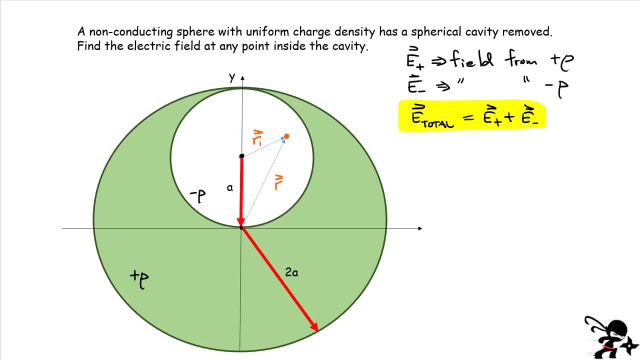 this right. so we're considering we're going to label e positive as the field due to a full sphere, green sphere that has a uniform charge density, positive row, and to that we have to add the field due to a negatively charged sphere. It's smaller but it has the same charge density. 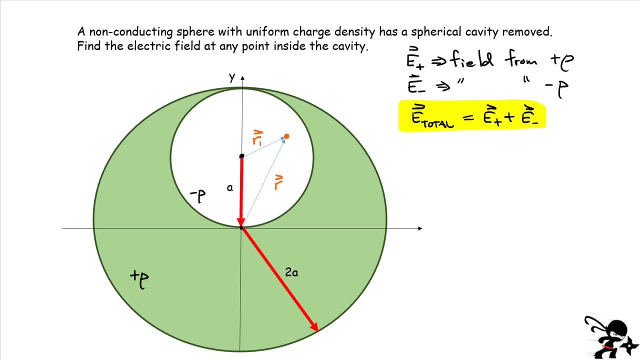 All right, and at the end, our total electric field. at any point I would write it as a positive field, and the total field has to be the vector sum of both of those. So let's go ahead and draw those vectors. So how would e positive look? Well, again, it is a sphere produced by this giant. 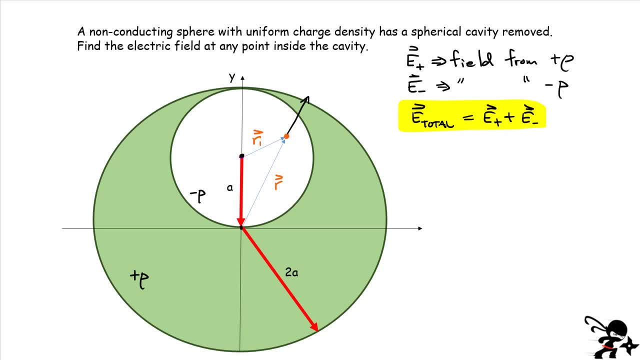 green sphere, so it should point away from it. in this direction, This would be e positive. Again, it points along the radial direction. All right. and what about the field produced by the negative charge density? Okay, well, that field should point toward the center of. 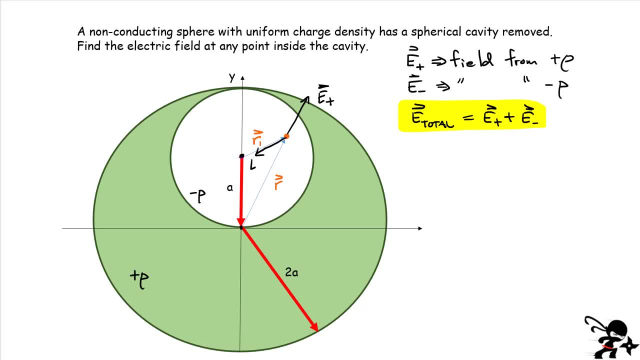 that sphere because it is a negatively charged object. So this vector here should look like this. okay, pointing toward it. Now I just saw in the first part of this video how do you find the magnitudes of each one of these? Again, they're just uniformly charged spheres, so you. 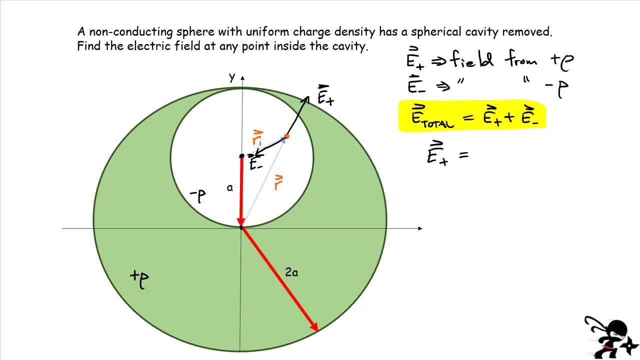 should be able to just write it down So that vector e positive- we can write exactly as I did in that previous case- multiplied by the vector r- Remember it's pointing radially away from the sphere center, E minus is pointing toward. okay, and that one looks a little bit different. Same charge, density. 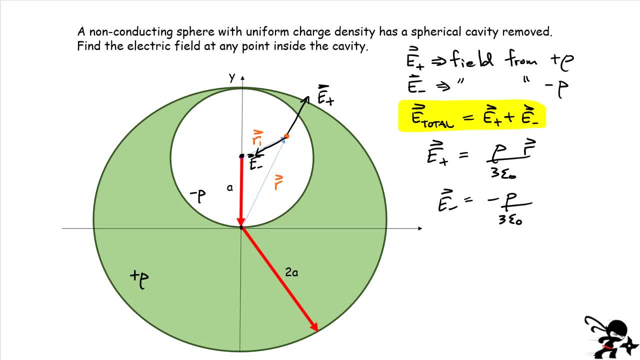 same factors over here: 3, epsilon 0.. Now the vector. you got to be a little bit careful, right. It points toward which sphere? It points toward the center of the little sphere. I've defined that vector as r1.. All right, these are not the same right. Clearly they're in. 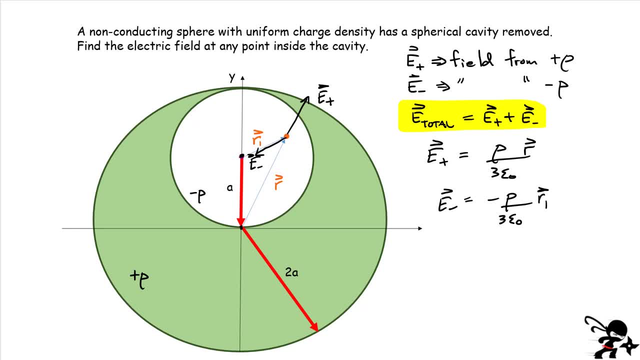 different directions. So we have to now look at this geometrical figure right here and we're going to link both of these vectors. So we're going to link both of these vectors and we're going to link both of these vectors together. all right, There has to be a link here between them. 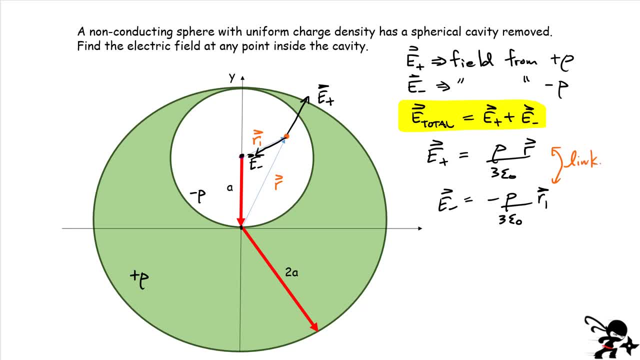 And the way that you can do that now is using this additional vector right, which goes from the center all the way to the edge. So I'm going to write down a relationship and we'll make sure it makes sense in a minute. So the link between both of them, you can write down the vector r1, which 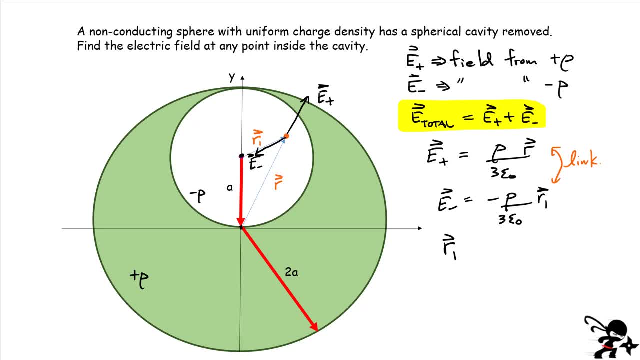 goes from here to there, right from the center of the small sphere to the point of observation. I can write that down as minus a times j. okay, a is the magnitude, that's the radius of the small sphere and it's pointing down. so that's this red vector. 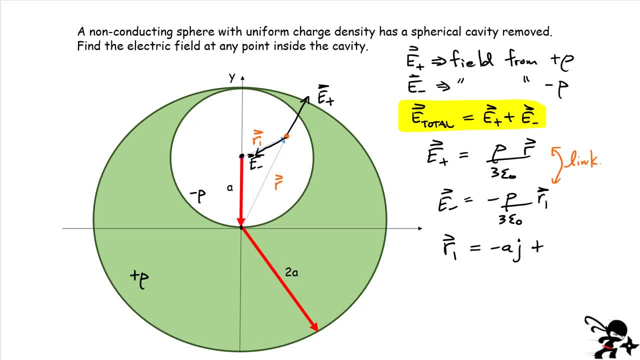 plus the vector r, r goes from the center of the big sphere all the way to the point of observation. All right, if you understand this equation right here, let me highlight that because this is an important one, Make sure you do. It's going to allow us to find the total electric field and 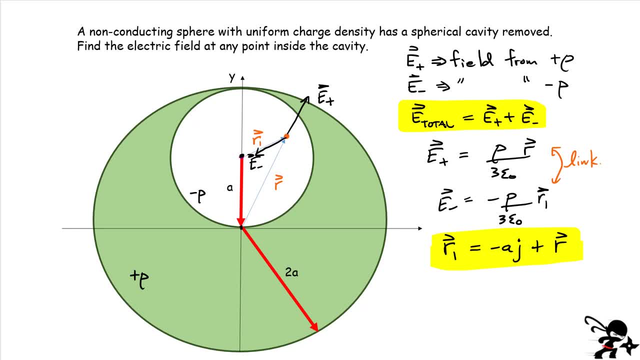 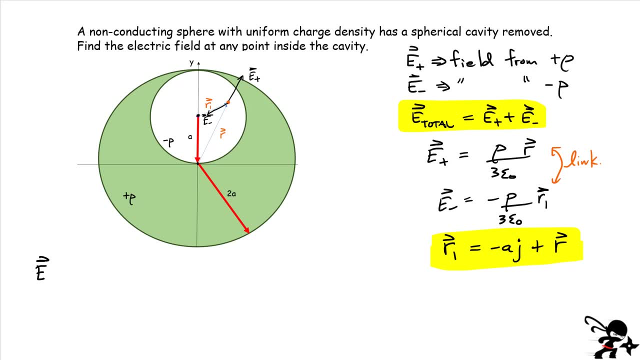 simplify this notation a little bit. All right, let's go to the last page and finish this problem off. All right, so to find the total field, we just apply the definition Our total field inside that cavity- again, it's that highlighted equation right here. so e positive is rho. 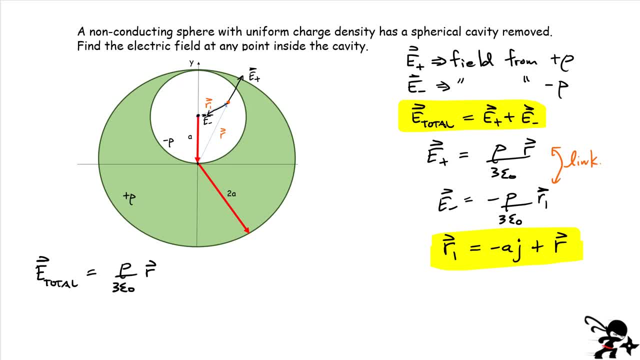 divided by 3, epsilon 0 multiplied by the vector r and plus the field due to the negatively charged smaller sphere. All right, and this is the vector r1.. Okay, now what you want to do is you want to take our definition of r1 and substitute it in here. So actually, 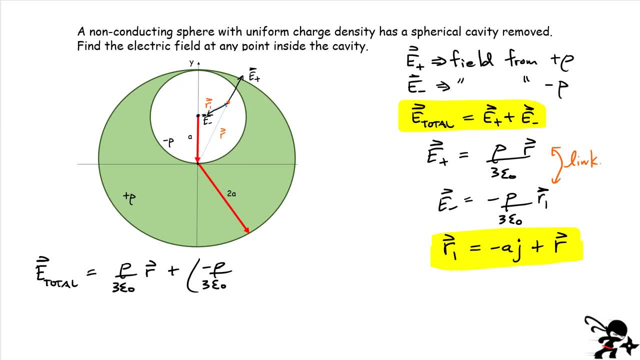 let me just get rid of r1 right here and replace it with this second term. This is minus a multiplied by j plus the vector r. Okay, now we have to do a little bit of algebra. Okay, you can see here that this first term